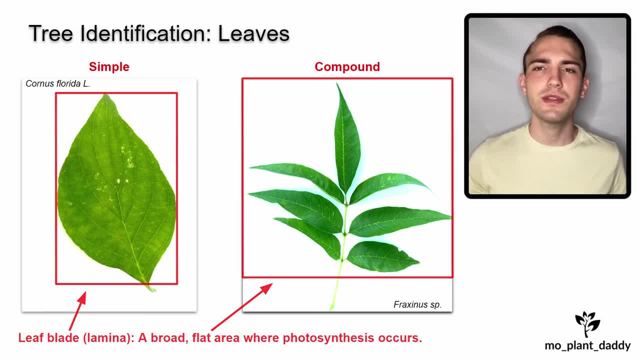 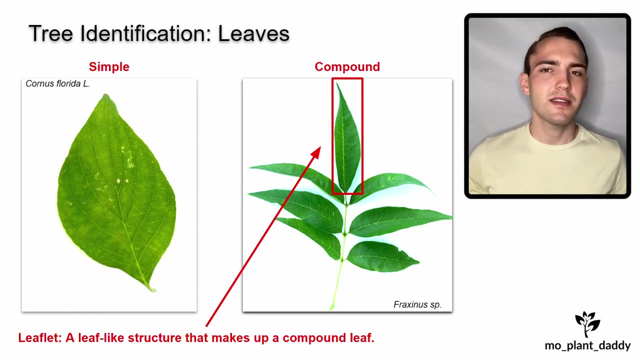 leaf. However, a compound leaf will have multiple small leaflets per blade. If you look at our example compound leaf, it has seven total leaflets. A leaflet itself is a leaf-like structure that makes up a compound leaf. Now, what about those little nubs there at the ends of the leaves, Those 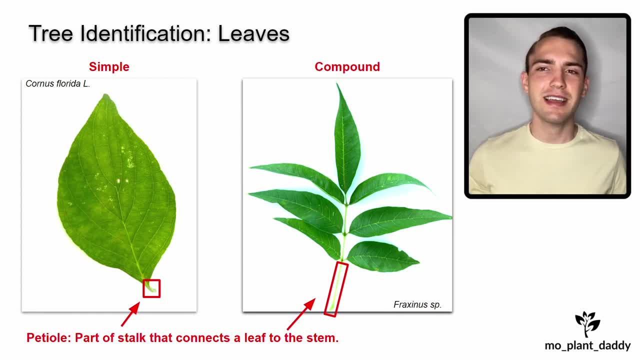 are the petioles, which is the part of the stalk that connects the leaf to the stem. Both simple and compound leafs will have three different iks. However, only compound leaves x2 have a rachis, which is the point on a compound leaf where the leaflets meet. 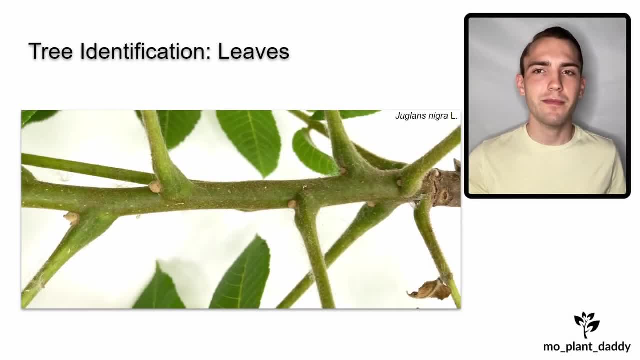 A helpful way to determine if you have a simple or a compound leaf is to look for a bud. hier we have a photo of the stem of a Jugland's nigra, otherwise known as a black walnut tree. In this photo we can spot multiple lateral or auxiliary buds, which are buds that reside on the side. 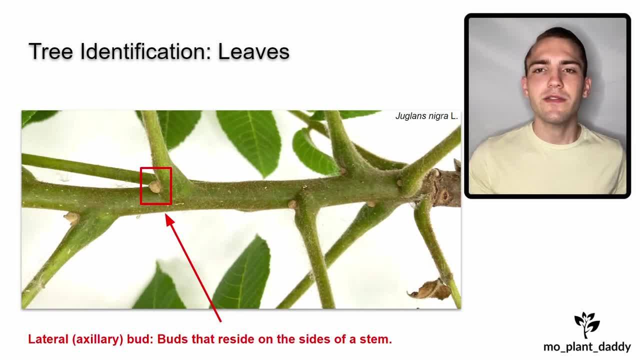 of a stem If a leaf is compound. all of the leaflets mixed with the anciparis sept 중에 are less受 Print E BY H. PROTECT philosophy, which shows that components can also be used for growing different leaves or vegetation. 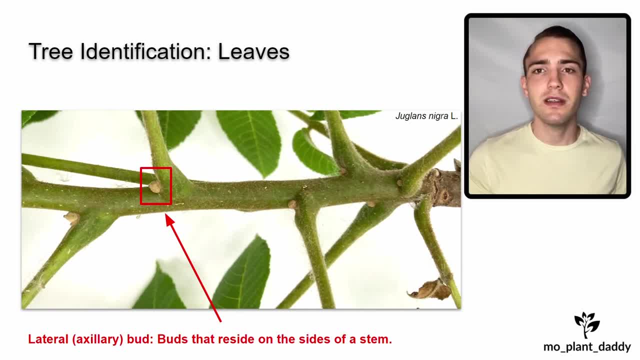 when you and your child are growing away from technology. Fitzp, mexican Style. A nice image is a 부�bling plant. if you're looking for a new plant, you can begin writing on your own will come from one bud. If you find a lateral bud, look at what is attached to. 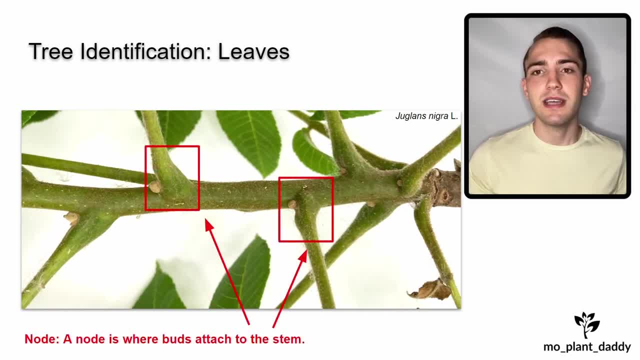 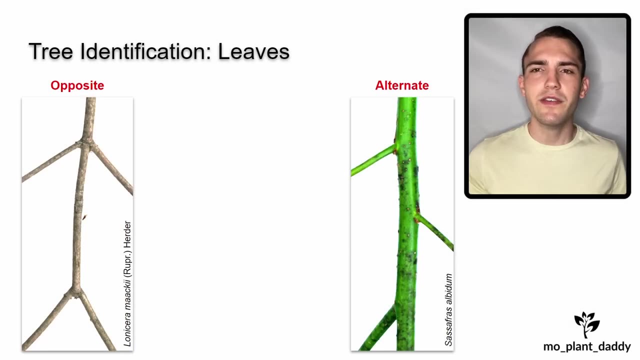 the same node as it. A node is where buds attach to the stem and the space between two nodes is called the internode. Any leaf attached to the same node will be either simple or compound, depending on what is supposed to come from that bud. Determining if a tree has opposite or alternate leaves is a very 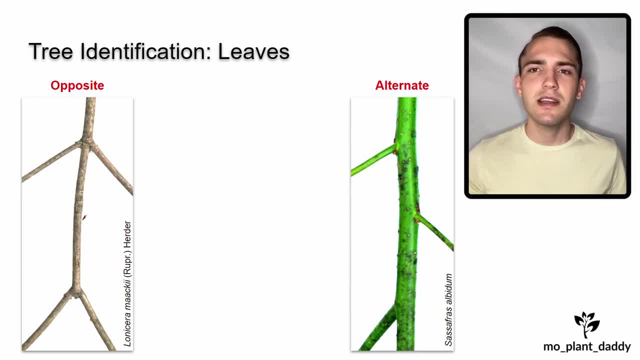 important step in species identification. Lonicera macki, otherwise known as a mer honeysuckle, is a species that has opposite leaves. An opposite leaf pattern is seen when two leaves arise from one node directly across from each other. On the other hand, Sassafras albidum, or the sassafras tree, has an 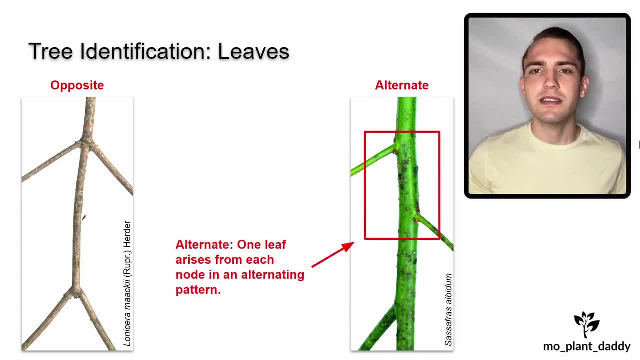 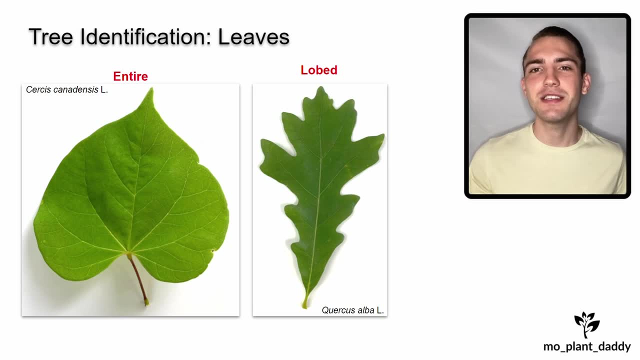 alternate leaf pattern. An alternate leaf pattern is seen when one leaf arises from each node in an alternating pattern. Okay, that's enough with the stem, so let's move on back to the leaves themselves. Let's start with leaf margins. A leaf margin is the outer edge of a leaf. There, 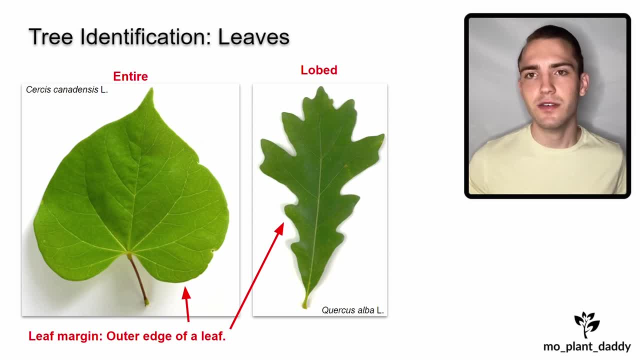 are two main categories. These are entire and lobed. Circus canadensis, otherwise known as eastern redbud, is entire, which means that its leaf margin has no lobes, Whereas Corcus alba, otherwise known as white oak, is lobed, which means that its 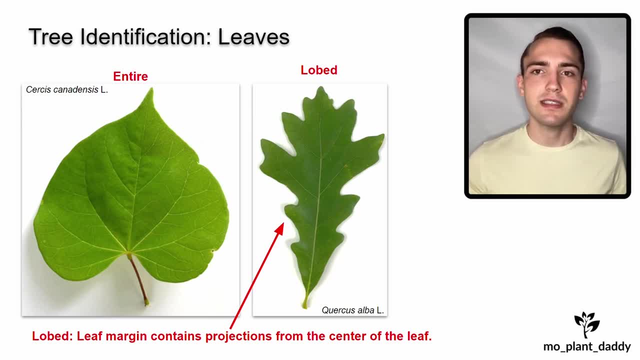 leaf margin contains no lobes. Therefore, Corcus alba is extended from the center of a leaf. Let's dig a little deeper into lobed leaves and talk about lobes and sinuses. We already know that a lobe is a projection that extends from the center. 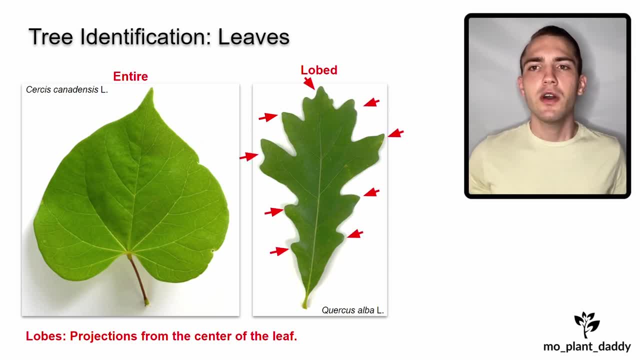 of a leaf. If we look at our Corcus alba leaf, we will see that it has nine lobes Sinuses. on the other hand, are the indents in the margin between two lobes. On our Corcus alba leaf there are eight sinuses, Besides being entire lobed. 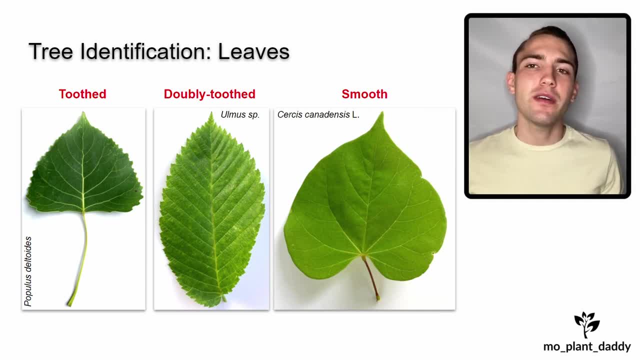 leaves can be toothed, otherwise known as serrate, or they can be smooth. When a leaf is toothed, its margin has a saw-like texture to it. An example of this would be Populus deltoides, otherwise known as eastern cottonwood. We can take this a step further and look at a leaf that 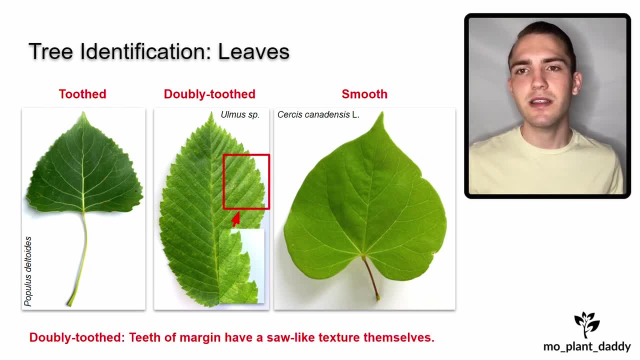 is doubly toothed. To be doubly toothed, the teeth of the margin have a saw-like texture themselves. An example of a genus with doubly toothed leaves would be Ulmus, otherwise known as elm. Lastly, for smooth leaves, there are no teeth present on the leaf margin. 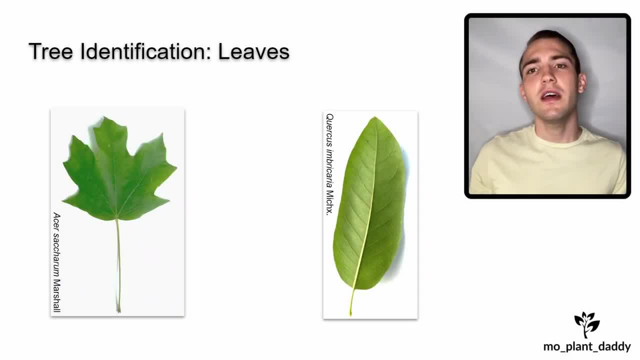 An example of this would be Circus canadensis. Veining patterns are also helpful in leaf identification because they influence the overall shape of the leaf. There are two main types of veining patterns for simple leaves that are super important to know. The first veining pattern is: 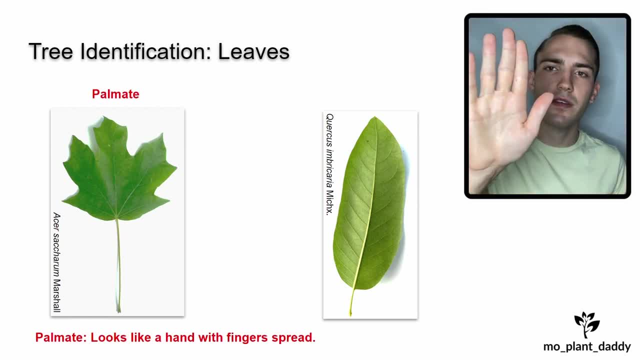 palming, which looks like if you were to put your hand out in front of you and spread your fingers. For other types of veining patterns, there are two main types of veining patterns. The first veining pattern is palming, which looks like if you were to put your hand out in front of you and spread your fingers. 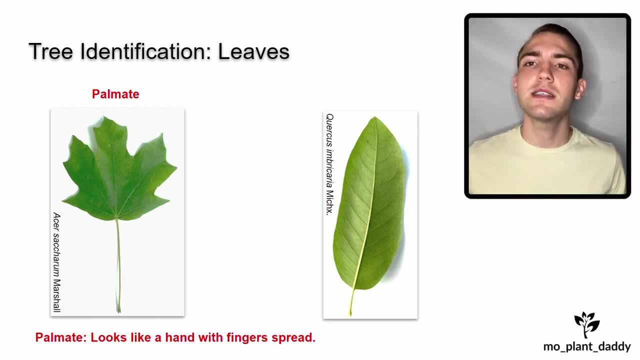 Acer saccharum, otherwise known as sugar maple, is a very well-known species that has a palmate veining pattern. The next commonly found veining pattern is pinnate, which resembles a feather and has similar parts on either side of its mid-vein. Quercus imbracaria, otherwise known as shingle oak. 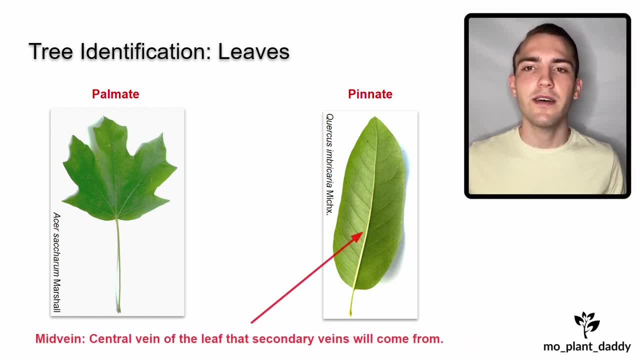 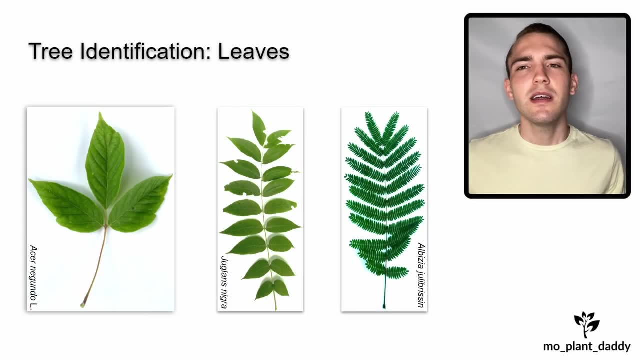 is a good example of a pinnate veining pattern. Now, the mid-vein is a central vein of the leaf, that secondary vein of the leaf, that is the central vein of the leaf. The secondary vein of the leaf is where the leaf's sediments will come from. Like simple leaves, compound leaves can also be. 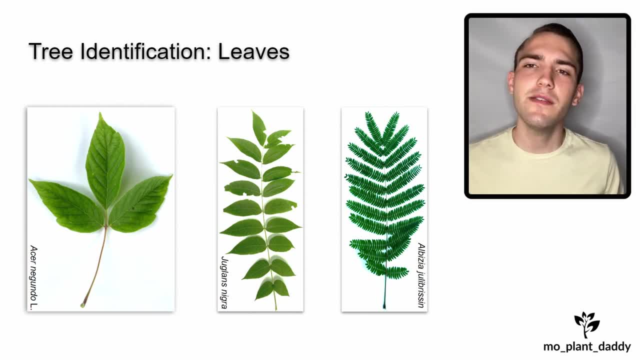 palmate or pinnate. instead of being connected, The leaflets make up the hand or the feather shape. Acer nigundo, otherwise known as box elder, is a fairly common species that is palmately compound, which means that all of the leaflets originate from one spot on the leaf. We can see that right. 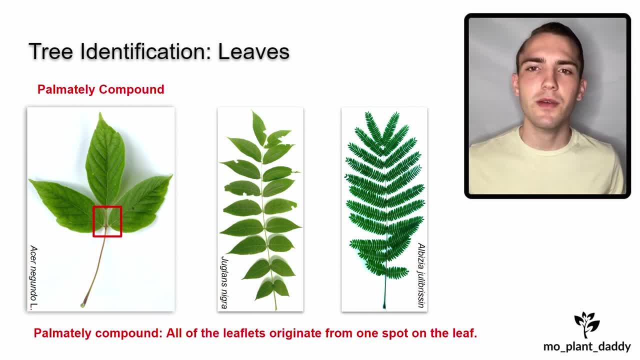 here. If we imagine this leaf as a hand, it would only have three fingers because there are only 3 leaflets- leaflets. On the other hand, Juglin's nigra or black walnut is an example of a pinnately compound leaf. Pinnately compound leaves have leaflets that are arranged on either side. 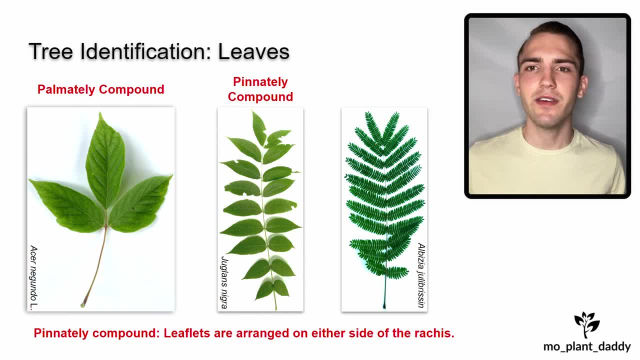 of their rachis. Now we can take this a step further, because some leaves are bipinnately compound, which means that each of their leaflets is divided again into even more leaflets- And I know that is a whole lot of leaflets. But an example of a tree that is bipinnately: 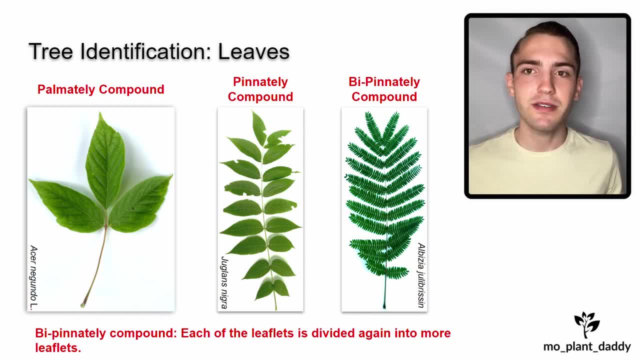 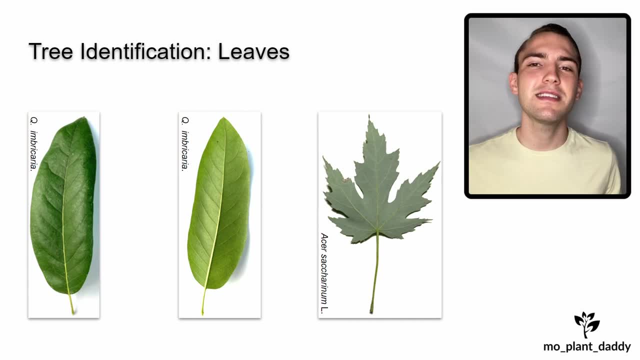 compound is Albizia jewelbrison or the mimosa tree. As we've seen, there are a lot of small ways to differentiate between leaves, but there is, however, another way. That way is to see if the leaf is glabrous, glaucous or pubescent. A glabrous leaf is one that 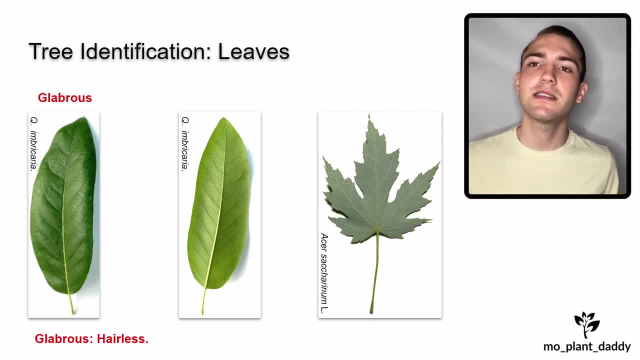 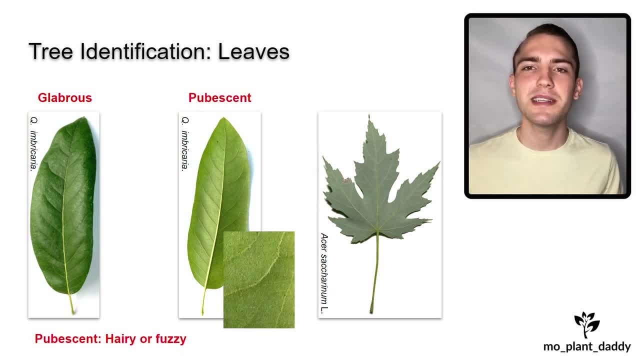 a corcus imbracaria leaf is pubescent, which means that it is hairy or fuzzy. Now that we're familiar with glabrous and pubescent, it's time to tackle glaucous. A glaucous leaf is one that appears bluish-white and waxy. An example of a glaucous leaf would be the. 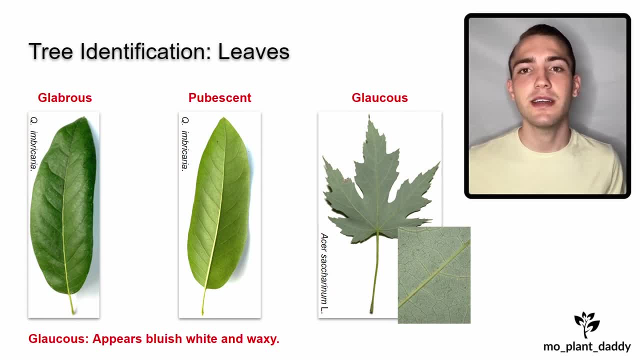 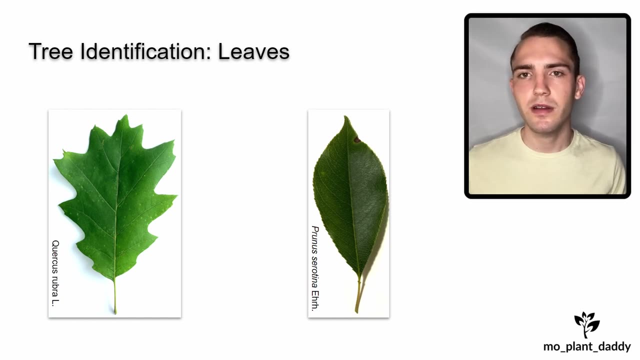 underside of an Acer saturinum leaf, otherwise known as silver maple, You can see that it has that palish coloration to it. Now there are some additional traits that leaves may have that we, as plant identifiers, could put to use. Some leaves like those of Quercus rubra. 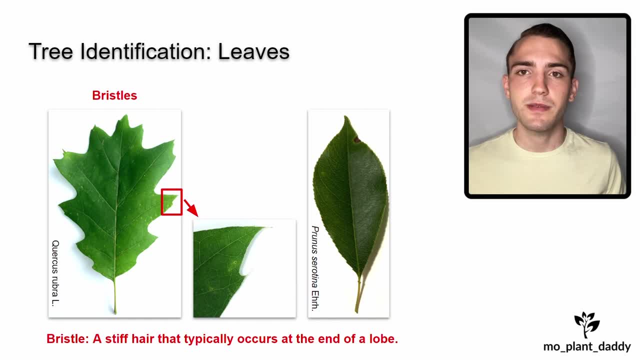 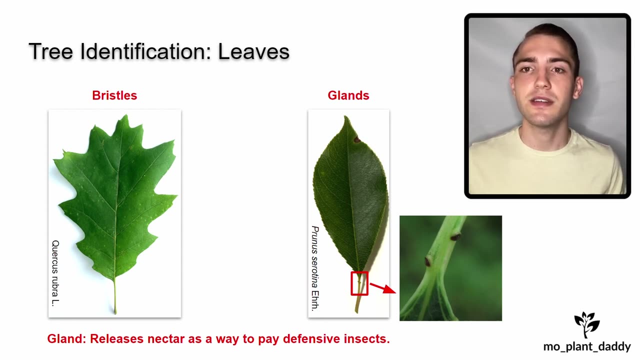 otherwise known as red oak, have bristles at the end of their leaves. A bristle is a stiff hair that typically occurs at the end of a lobe. Another trait that is less common is glands. A species in my area that has glands is Pruniceratina, otherwise known as black. 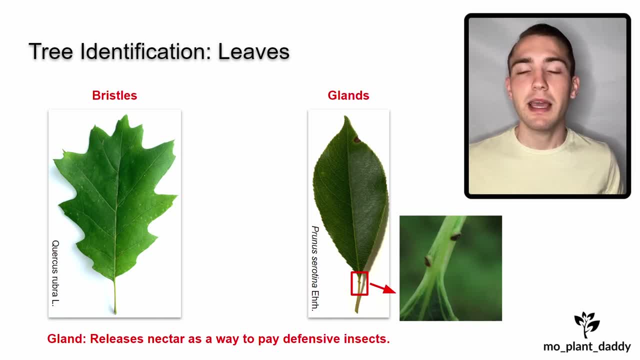 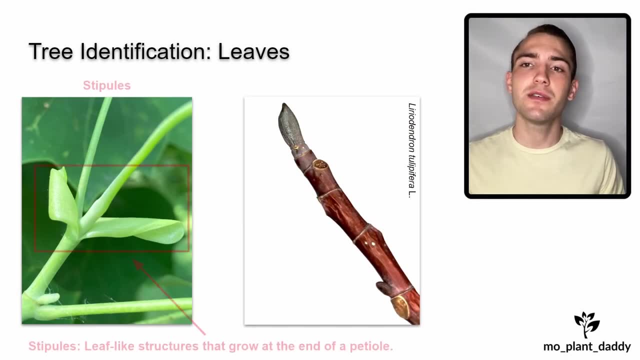 cherry Glands release nectar as a way to pay insects that eat herbivorous insects that can be harmful to the cherry tree. Lastly, stipules are a pair of leaf-like structures that grow at the end of a petiole. The stipules pictured are that of Liriodendron tulipifera. 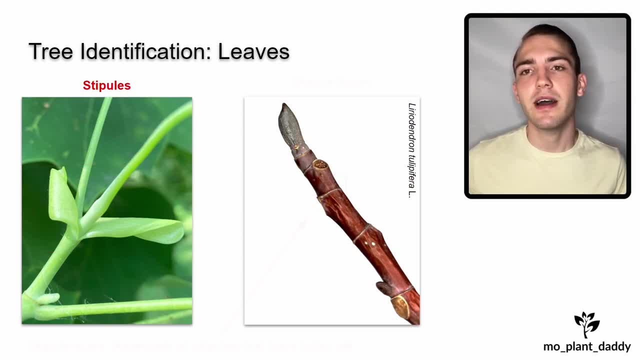 or the tulip tree. After they fall off, they leave behind a stipule scar and in this case it will be all the way around the twig of the tree. This can be useful for identifying the twig in the winter time. But ok, just for funsies. we're going to do an example Here. we have an unknown tree species in front of us. We'll be однаwoing them next week, but make sure you a long and careful test in this video. 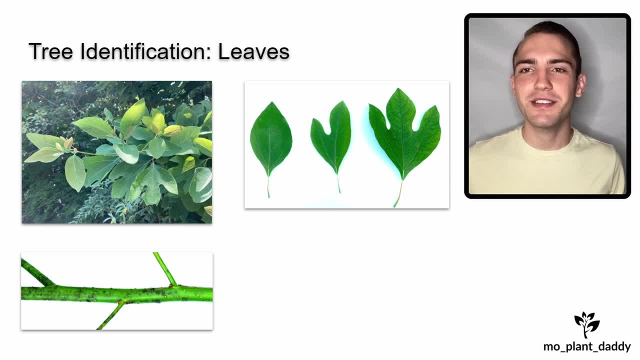 Here we have an unknown tree species in front of us. We'll make sure you a long and careful test in this video. Please keep that in mind. to do an example: here we have an unknown tree species and some of you might already know the. 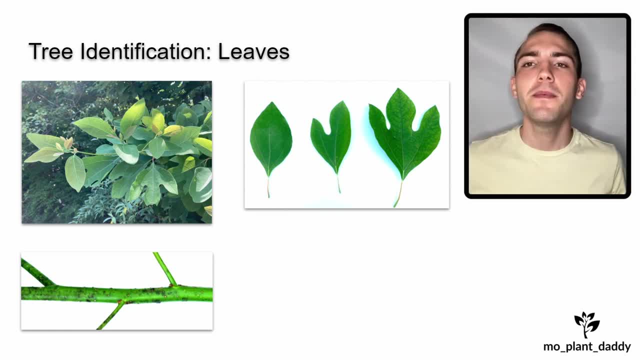 answer- but please don't shout it out because that would be kind of rude- but we're going to work through a series of questions to review what we've learned and together we are going to identify this tree. so there are six main questions you should keep in mind when you are identifying a tree. 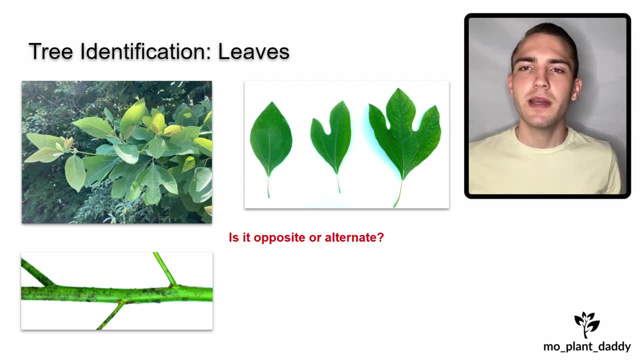 the first being. is it opposite or alternate? based on the section of the twig shown here, we can safely say that it is alternate, because the leaves are attached in an alternating pattern. are the leaves simple or compound? they'd be simple because they are not broken into leaflets. 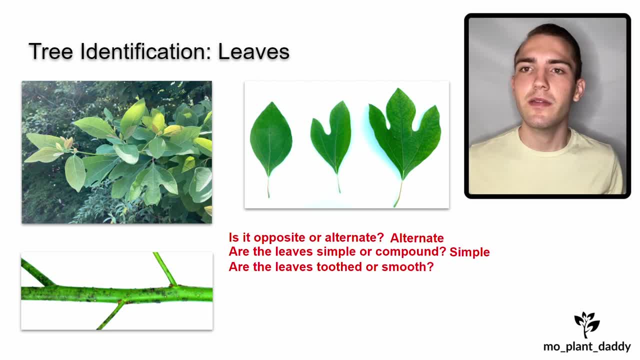 are our leaves toothed or smooth? they are smooth because the margin of the leaves do not have a saw-like texture. are the leaves lobed or entire? these leaves are lobed. this particular species is innocent and they grow heightlessly depending on what type of leaf they own. if they grow too, out of thickness. they areэ strange to soothe them. similarly, if they grow tall, if they grow too flat, if they grow too thin on theDeser or off, they grow not enough and they build thin for a tree. 100% of them need more of the leaf size and there can be some stop and the trees make a ton of. 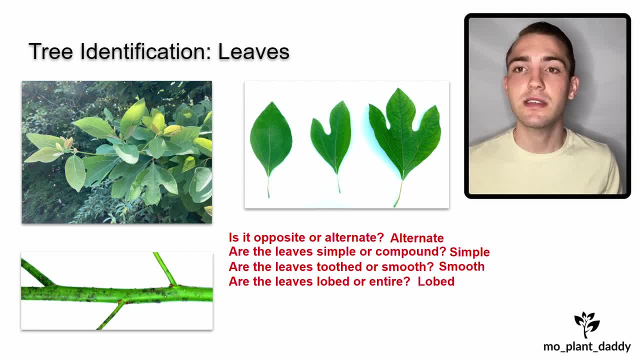 ience. also if you see some trees in the potential to expectおuh if the leaves become at least 20%, and if we look, because there's three different types of leaves. The first is single lobed, which could be classified as entire, but it also has a two lobed and a three lobed.